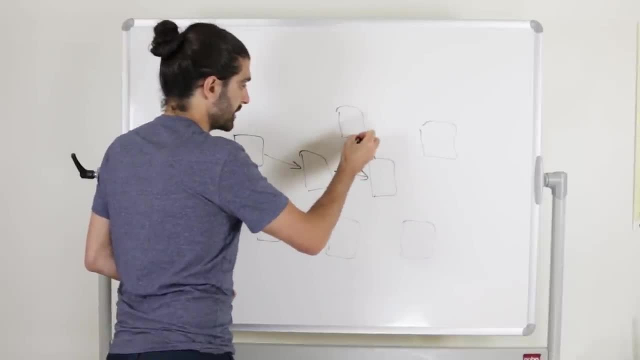 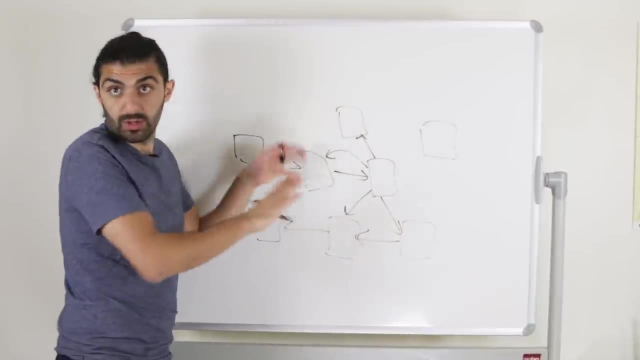 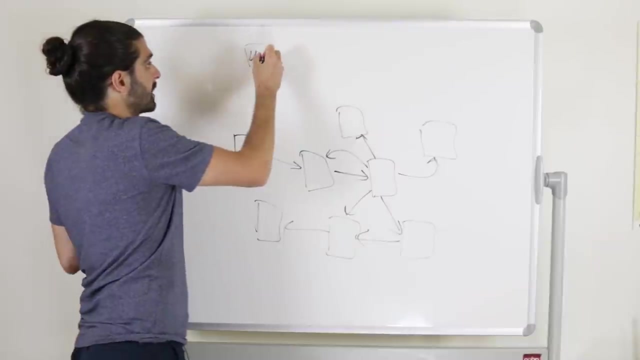 this uses this and this uses this, but this one uses this one and this one actually also uses this one, and this one uses this and this uses this, And then you've got a client. and, as usual, when we say client, we don't mean client as in customer. 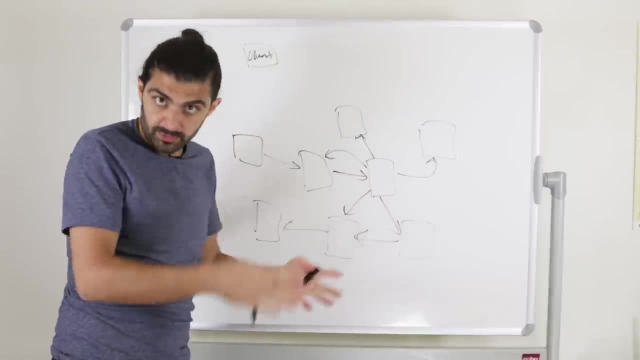 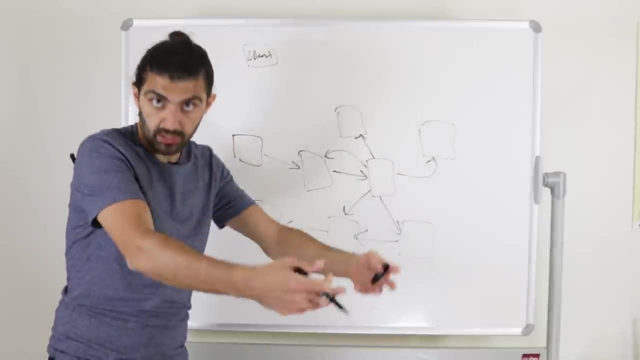 we mean client as in a user of a particular piece of code. In other words, not a user as in an end user, but a user as in a particular piece of code using another particular piece of code. So here's a piece of code that wants to use some pieces of this code, And the point is that this kind of 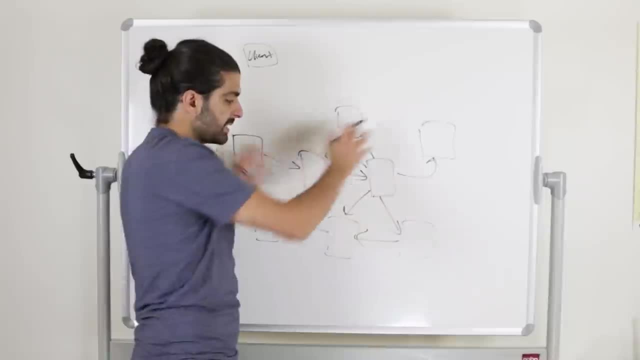 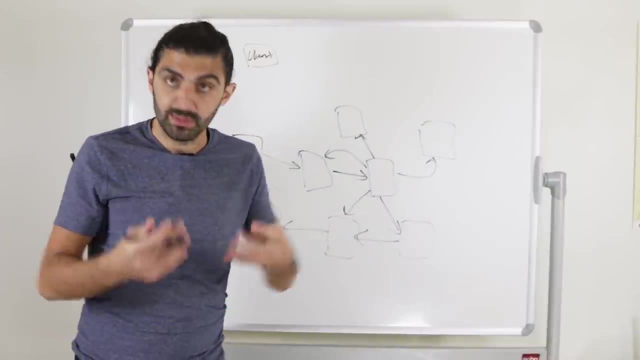 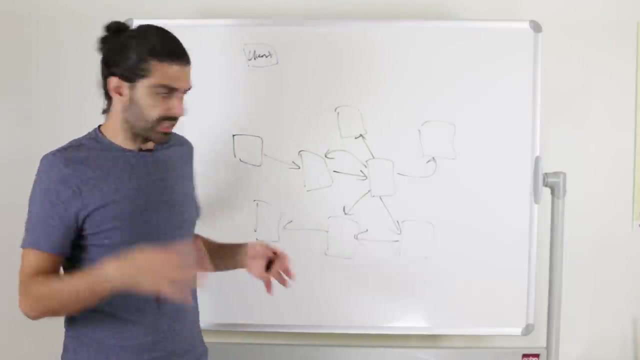 client wants to use these different pieces in some particular manner. The reason that something might look like this is that we might have an extremely decoupled system, So this might actually be a very good thing- probably not given this diagram, but I'm trying to say that you can have. 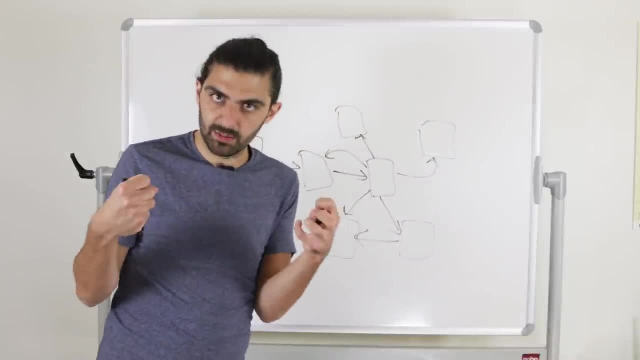 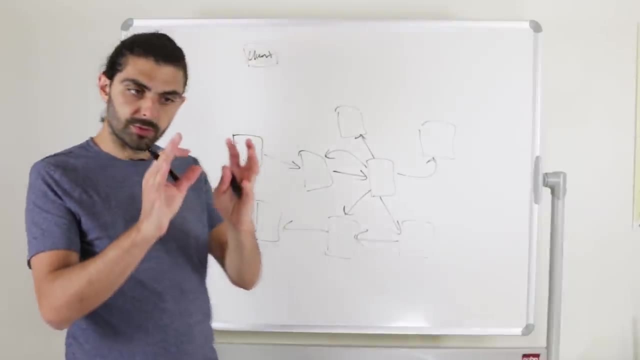 lots and lots of classes, even though you have a high decoupling. Actually, my spontaneous guess if you have lots and lots of classes would be that your system is highly decoupled because you have lots of classes that decouple. So if you have lots and lots of classes that decouple, 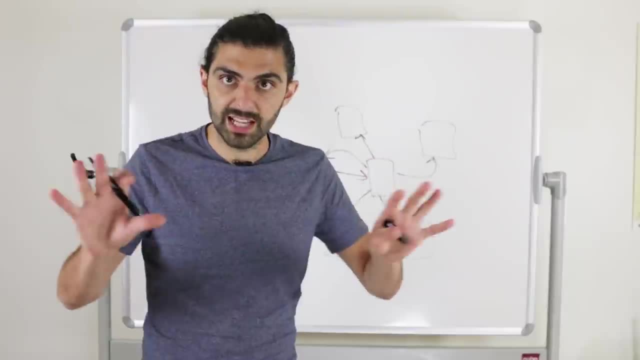 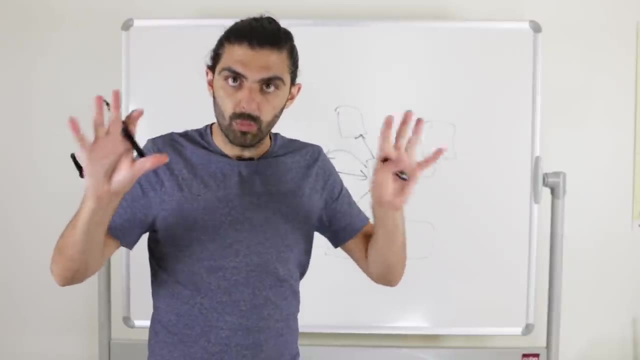 you have lots of classes that do lots of small things, Or sorry, I should say, you have lots of classes that each do a very small thing. So, single responsibility principle, right, Each of your different classes do one thing and one thing only. And if you keep following that principle, 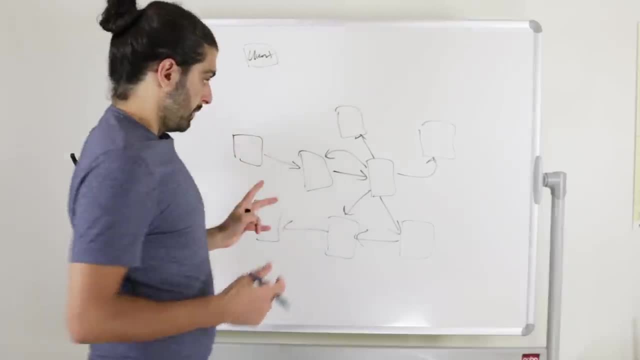 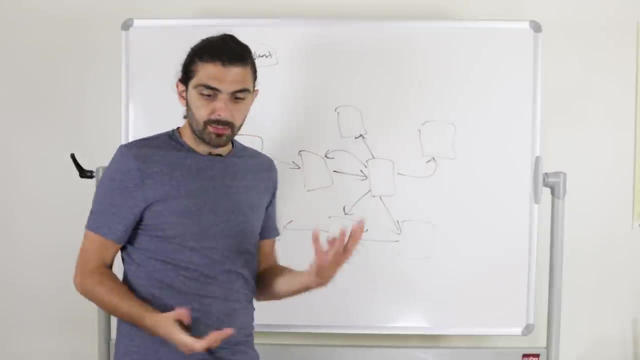 you'll end up probably with lots of different classes. Now that means sometimes, when we do this, depending on the complexity of the task, you might end up with lots of classes A and then B, having to use many, many classes in order to actually do anything meaningful. So 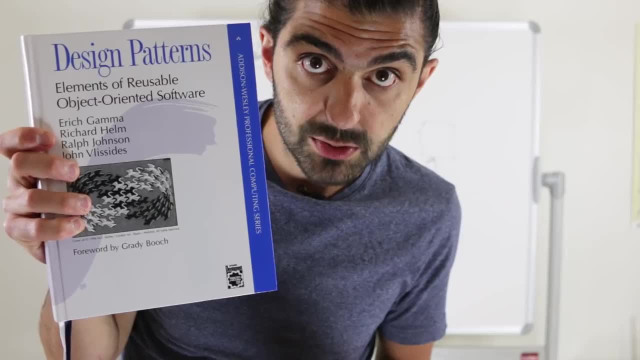 there's a lot of different ways to do this, And I'm going to show you how to do this. So let's start with the first one. So let's start with the first one. So let's start with the first one. Here's an example in this book: Design Patterns- Elements of Reusable Object-Oriented Software, by. 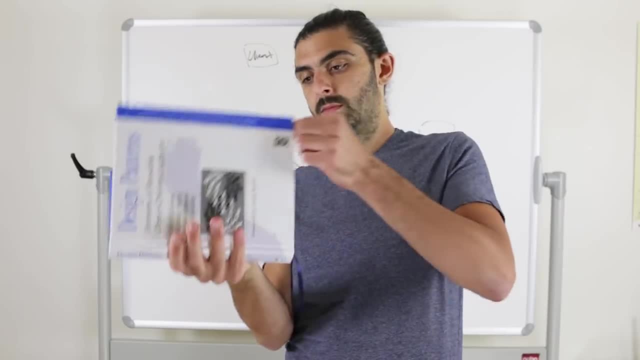 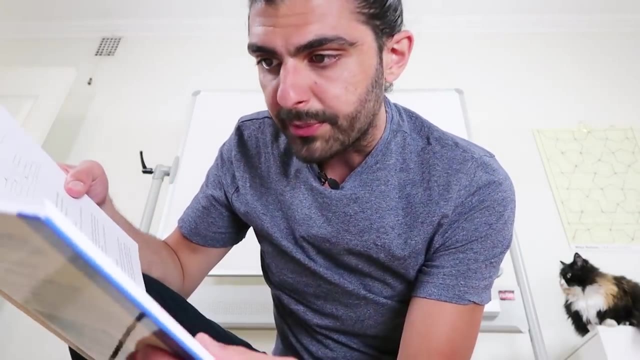 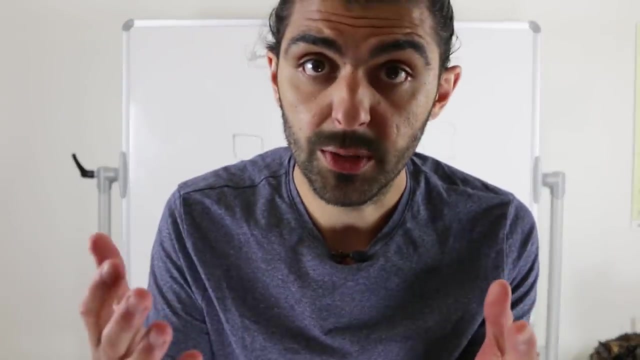 Gang of Four, When they talk about facade pattern, they have this image of a compiler. So there are a bunch of pieces from a compiler, like a scanner, a parser, token symbol, all of this stuff that you would probably use if you were building a compiler. So in other 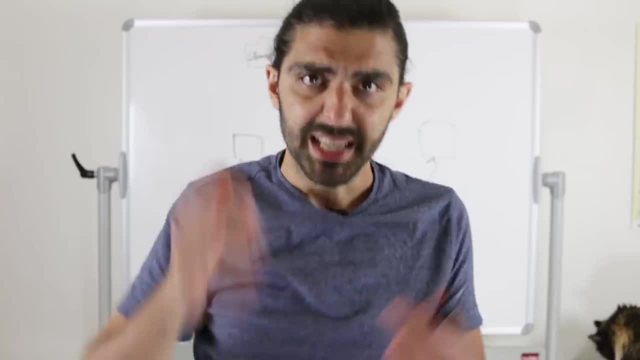 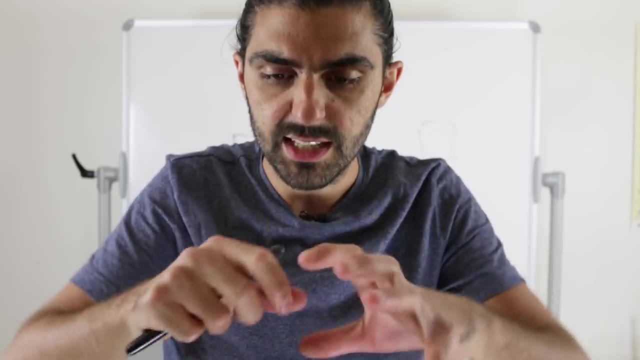 words, a bunch of classes that you would probably use if you were building a compiler In. even other words, it would make sense to divide, to structure up your program in these different classes. In other words, it would make sense to separate things into these. 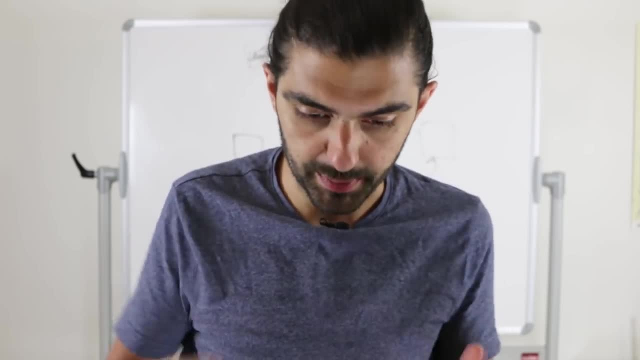 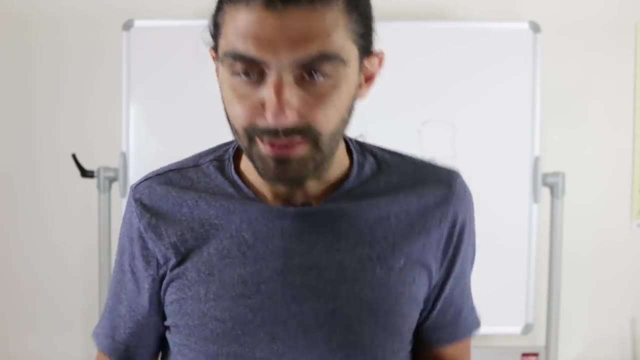 different classes, not necessarily these particular classes, but I'm emphasizing, it would make sense to have this high level of abstraction, It would make sense to separate to this extent. But, of course, when you do this, that means that in order to actually do any useful work, in order to actually 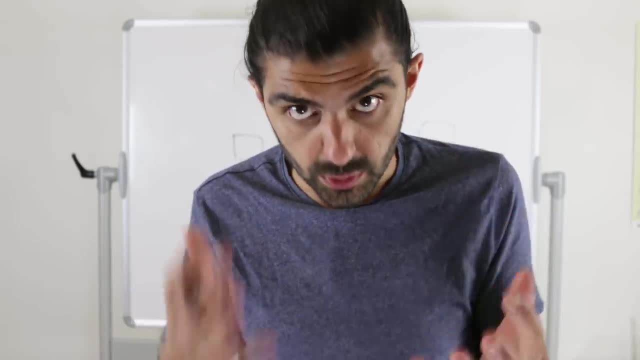 do any compilation of programs or whatever the task is that you are modeling, it might mean that you need to use lots of different things. So let's start with the first one. So let's start with the first one. Let's do not 191 classes at the same time, which can actually get kind of hairy. 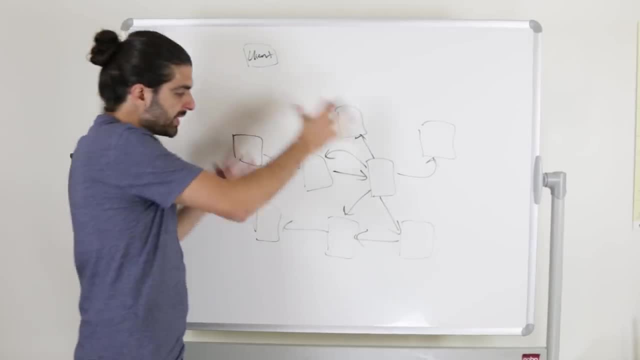 which is exactly what we're looking at here, right Like? so, depending on how this is structured, right like, let's say that if this thing needs this thing- I'm not drawing UML now, so forgive my sort of informal notation if this thing is using this thing, but this thing is. 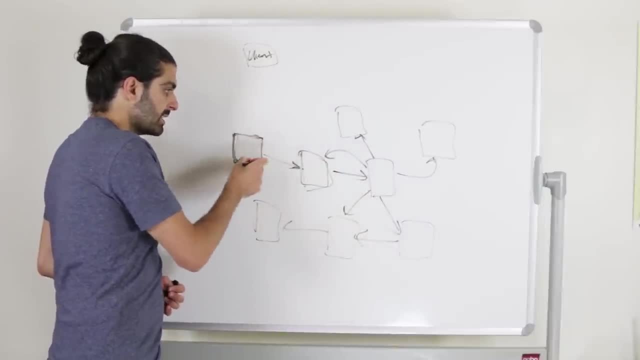 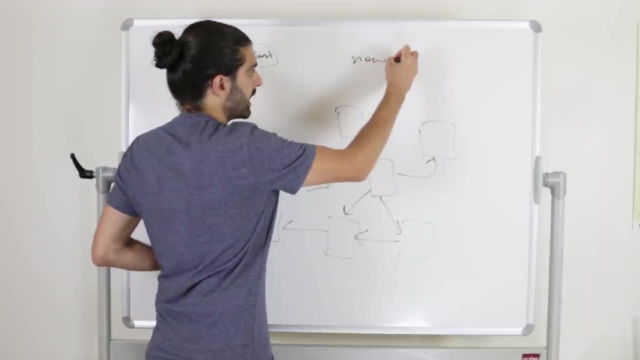 dependency injected. that means that in order to instantiate this thing, we needed to pass it one of these right. so let's say that this is a and let's say that this is b. So in order to say new a, we need to pass it a new. 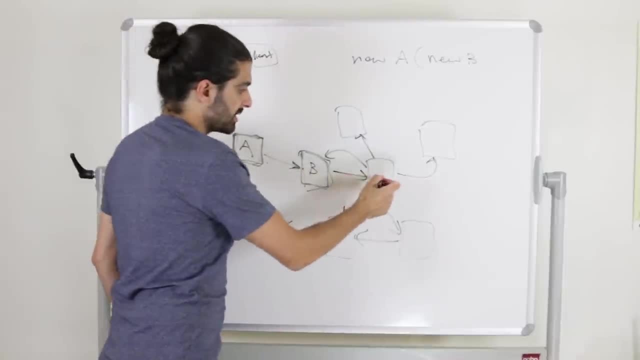 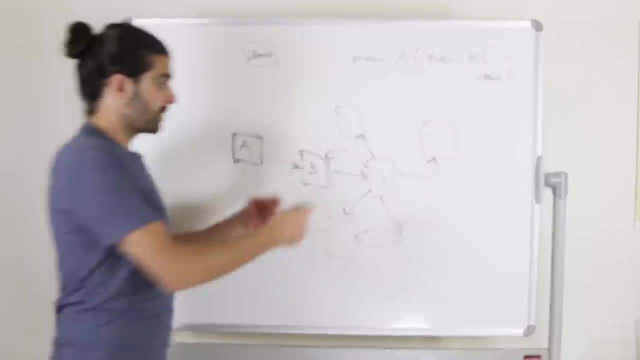 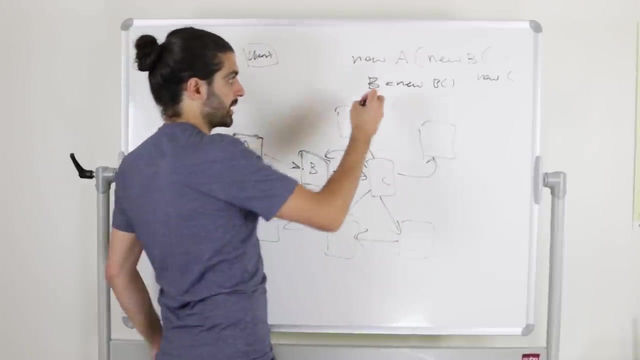 b, for example, but let's say that b's actually require c's, so new c. but actually that doesn't work because c needs a reference back to b. okay, so maybe it's even something more confusing. so it's like we construct a b equals new b, and then we're not passing c in the constructor, but we're 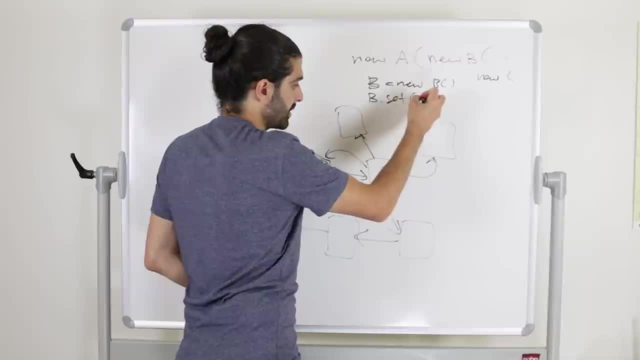 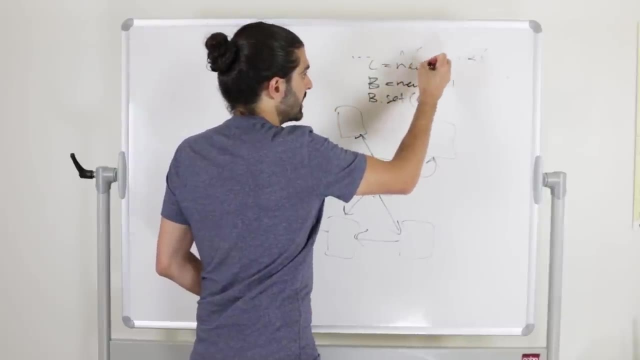 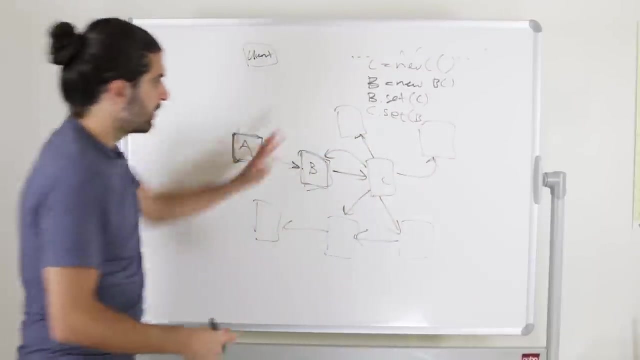 setting b. so we're saying like b as set, and then we're setting the c because that when we've also constructed the c before. so it's like c equals new c, no arguments, right. and then, and then on c we set b right. so it's like that relationship, something along those lines. i mean, i'm just doing. 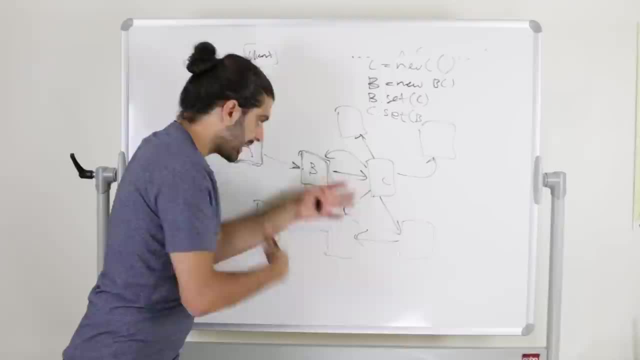 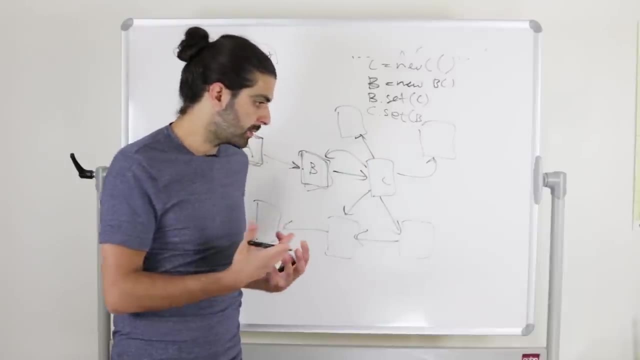 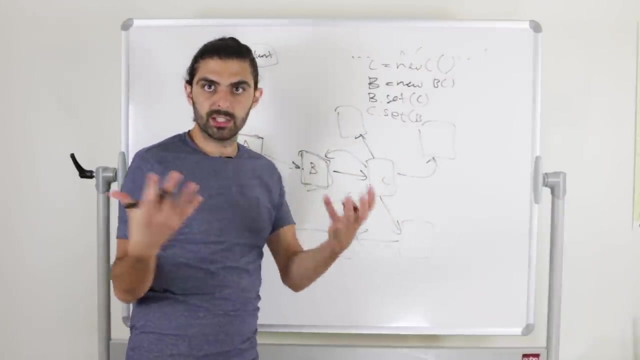 stupid stuff in order to show that, depending on the scenario, you might have a lot of difficult wiring. let's say right, like, depending on your scenario, it might be, or depending on your model, it might be non-trivial to to set up the data structure in the way that you actually want them set up in order to actually do any useful work. 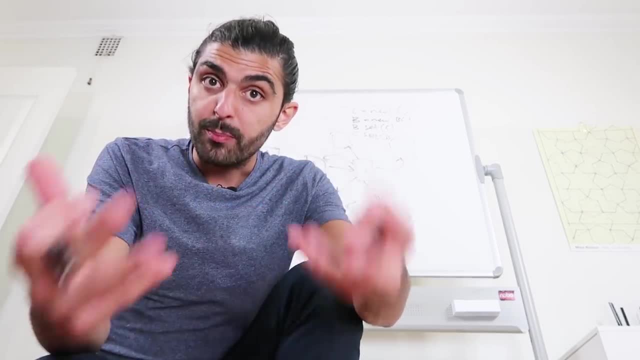 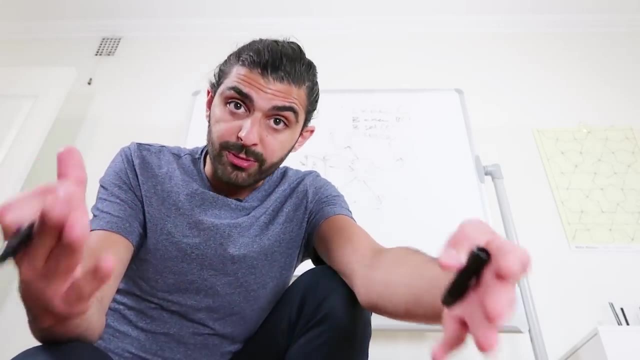 And that's fine. I mean, what we're saying here is not that that's a bad thing. I mean, having highly decoupled systems is a good thing, And having sort of complex setup might be, I would venture to guess, is almost a natural consequence of having highly decoupled systems. 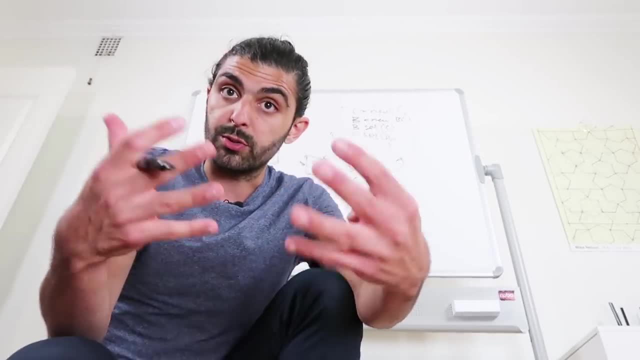 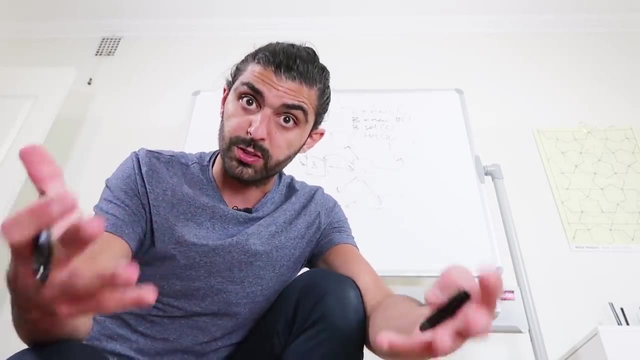 because you have very general pieces that you compose together in order to do useful things, But because they are so general, they can be composed in a multitude of different ways, which means that you can do a multitude of different things. So what is facade pattern? 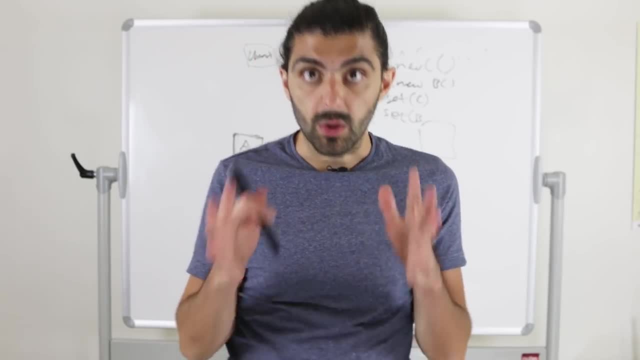 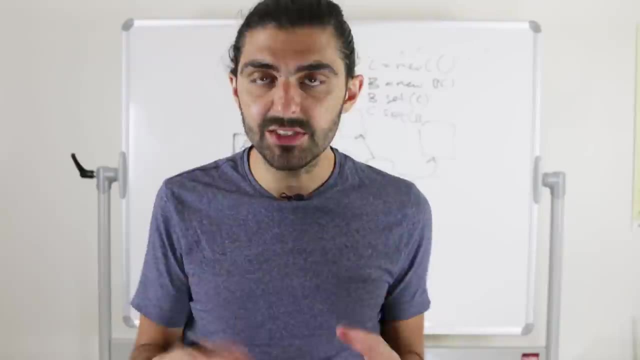 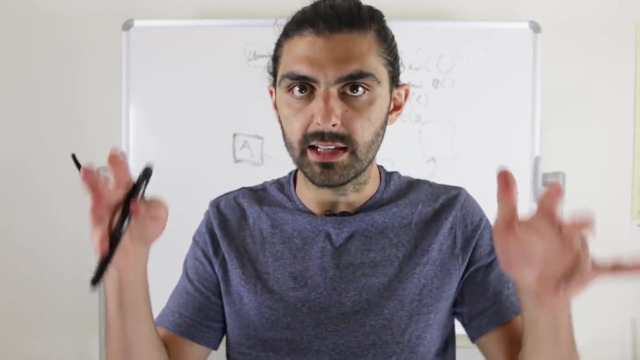 Well, facade pattern is a way of saying that. okay, it's fine that I need to do all of this complex wiring, But if I'm going to do this complex wiring, I want to have an easier way of doing it, And that's the facade. If you think about the word facade, the facade is the sort of 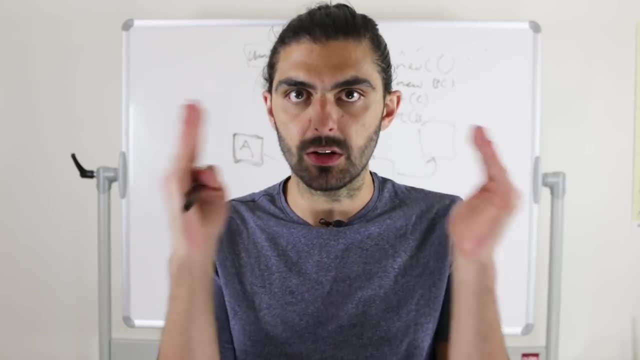 exterior of the building And if you think about the word facade, the facade is the sort of exterior of the building And if you think about the word facade, the facade is the sort of building, like the outside, the face of the building, And actually that's a very useful 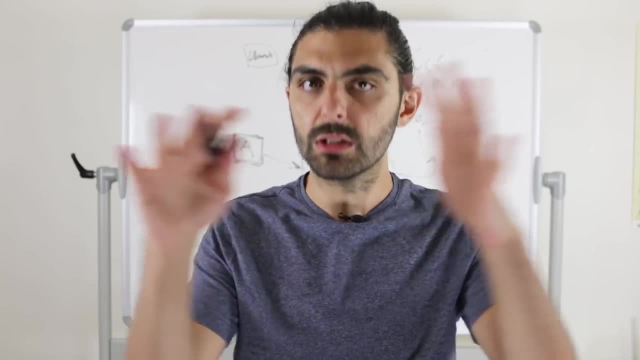 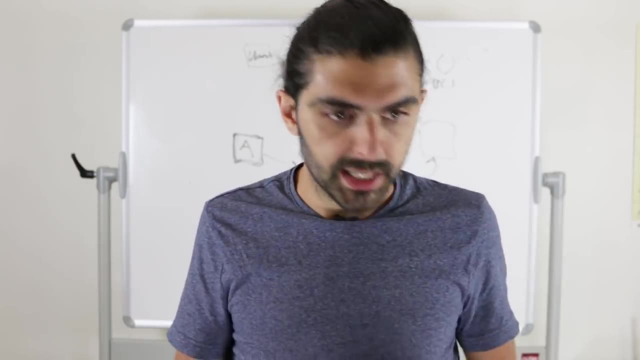 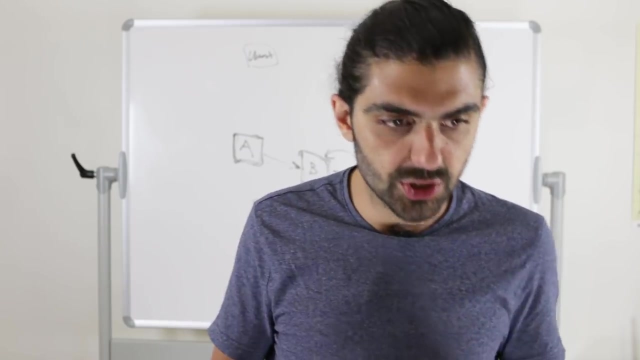 metaphor, because obviously the house is a lot, lot more than just the facade. If you just had the facade, it would be completely pointless. You need all of the plumbing and the. well, I know too little about houses, but you would need all of the plumbing and the isolation and the foundation and 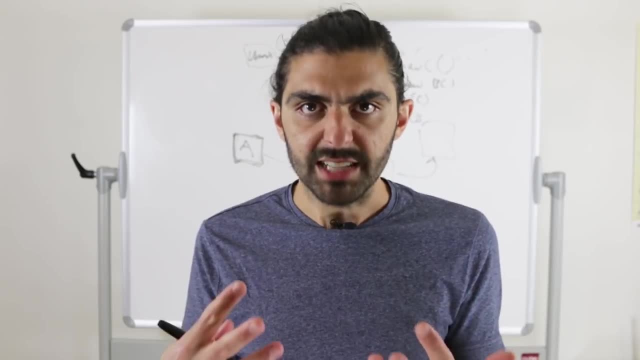 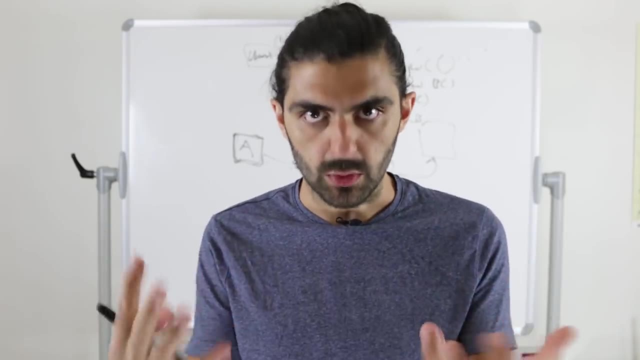 the wiring and the roof and, like all of all of that stuff, You need that stuff in order to actually construct the building. But then you also need the facade, because you don't want to be looking at all of the plumbing, And that's exactly what this is, the facade pattern. With the facade pattern, 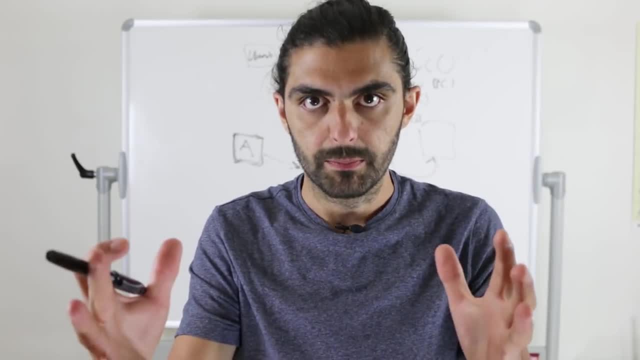 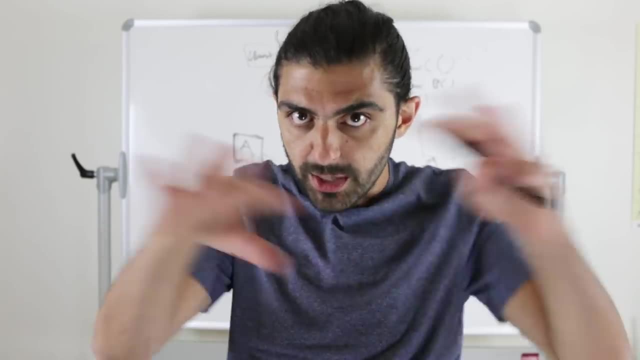 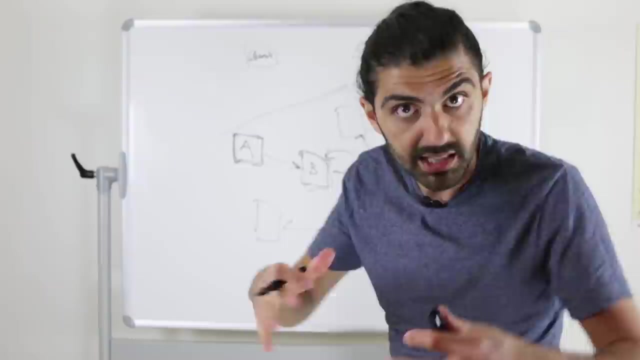 we're saying, underneath the facade we have a lot of plumbing, this stuff, But outside I don't want to have to deal with all of that plumbing all the time. So I'll create a facade right. I'll create like a nice wrapper, a nice interface that I can interact with instead like the face of the house. 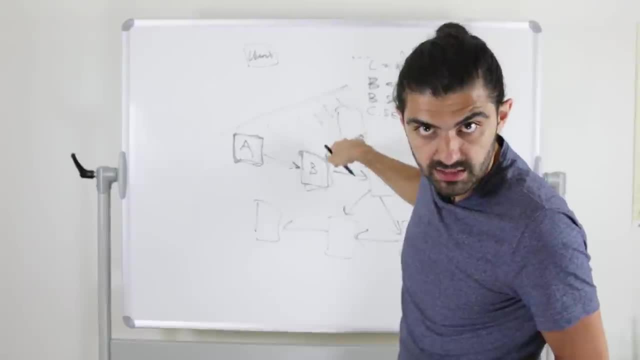 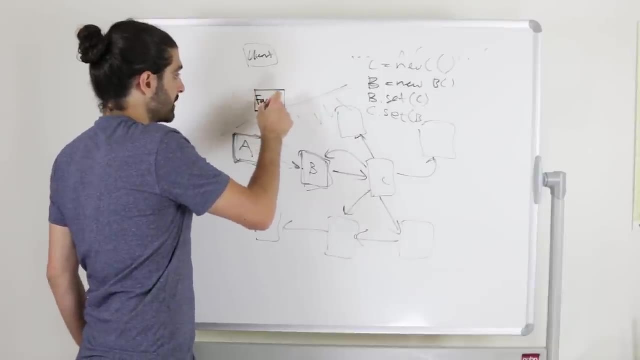 And that thing then interacts with all of this complex stuff, That interacts with all of all of the wiring. So if we're trying to draw this, that means we have this facade here, facade that the client interacts with, And then 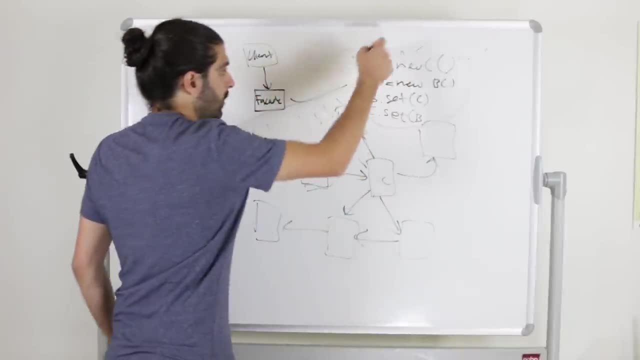 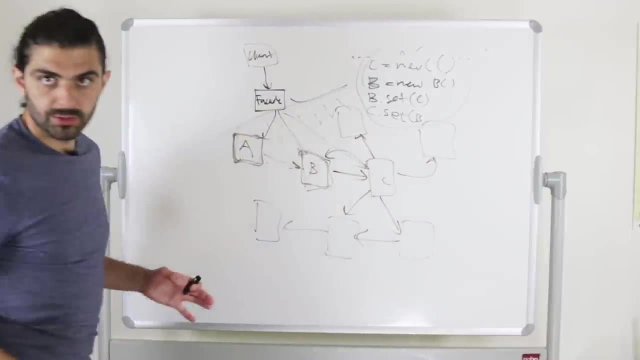 the facade does all of this stuff right. It does all of the complex wiring, whether that be, whether that starts with B and A and C or whatever that starts with. So I could draw a UML diagram, but really the UML diagram is just. 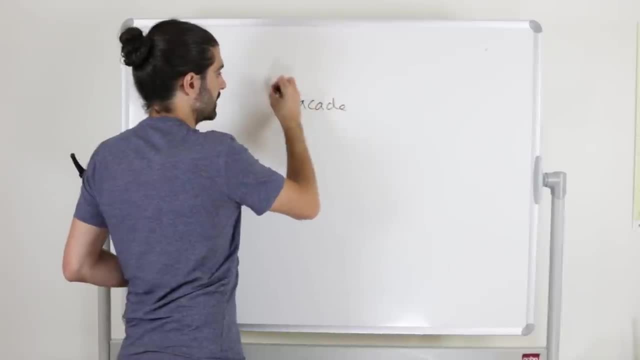 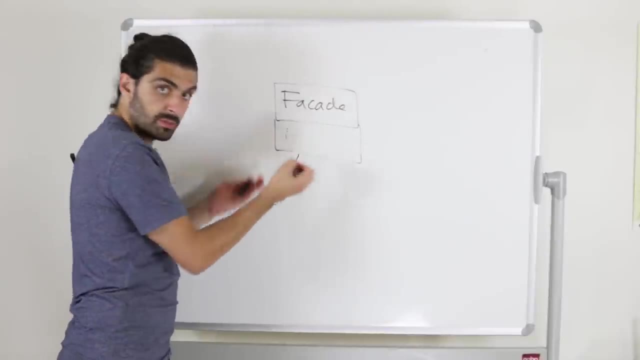 all the same thing is: it's just this. it's just a facade, is a class that has some set of methods And what it does is that it invokes methods on all just the dashed lines here to indicate that it could be any number of errors. 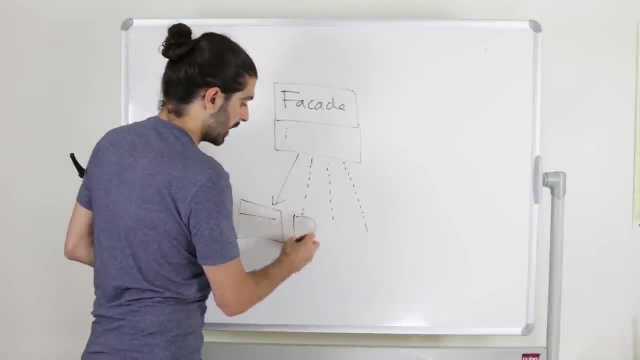 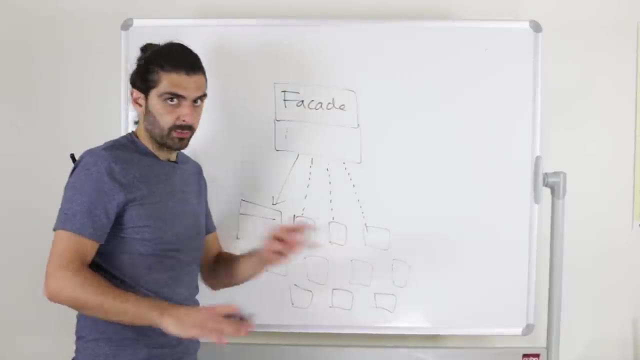 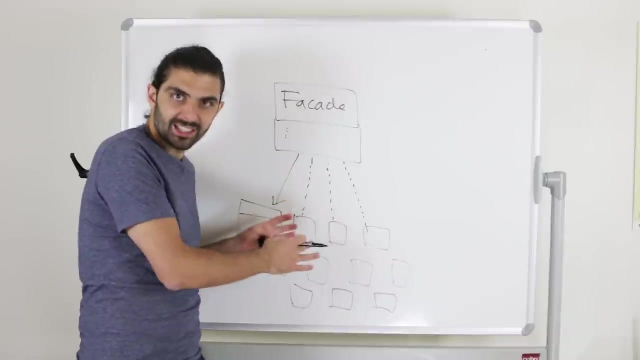 here. it invokes methods on a bunch of other classes. who invokes methods on a bunch of other classes, etc. etc. I mean, this is not composite pattern. we haven't talked about composite pattern yet, but it but it's not composite pattern. There's not some order to this madness, It's just madness. The thing that the façade is. 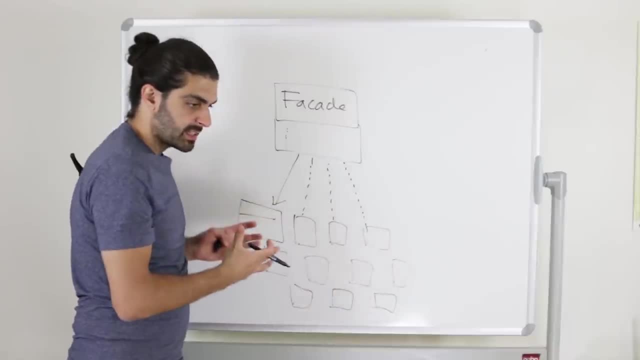 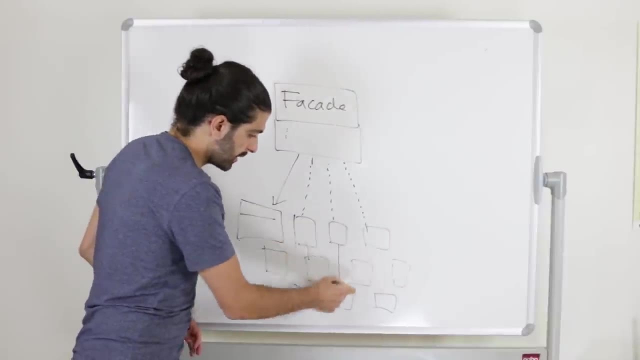 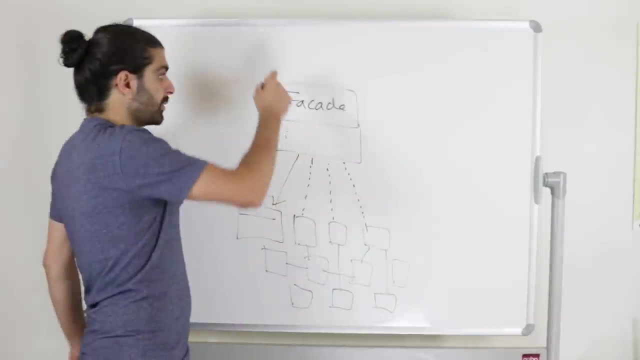 a façade over that stuff isn't necessarily following any particular structure. This stuff is completely dependent on your scenario. Sometimes you have arrows going this way and sometimes you have arrows going this way and, like, completely depends on your scenario. The point is that you construct a façade that interacts with these objects and simplifies the interaction, for 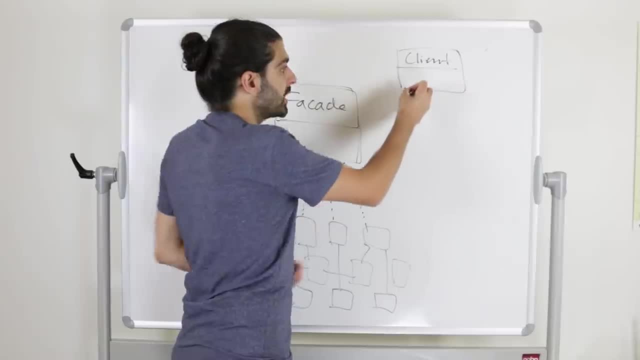 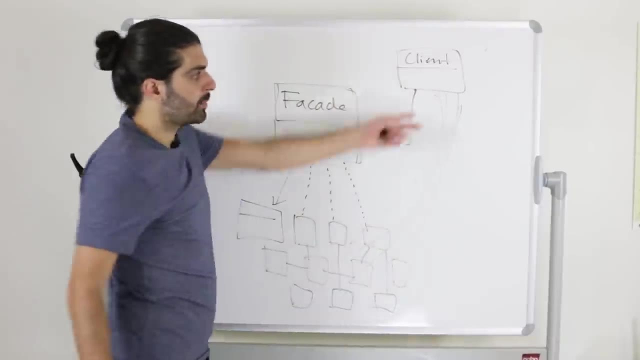 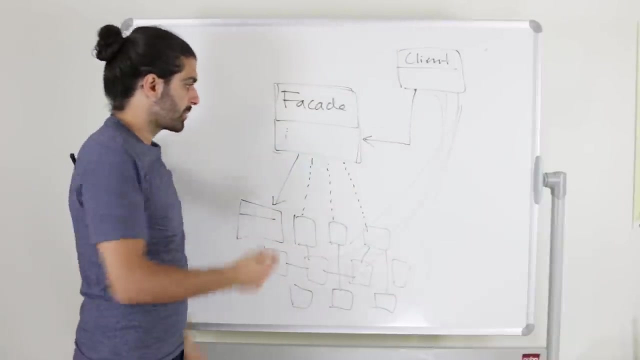 you so that when you have a client class, you can use this façade instead of having to directly interact with all of this stuff. And if you imagine that you have multiple clients, if you imagine that you want to do this complex interaction in multiple different places of your program, it would of. 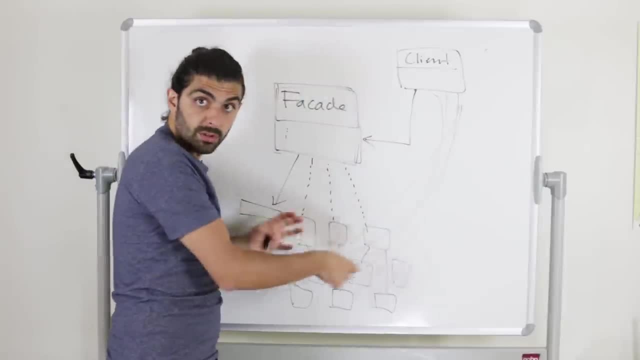 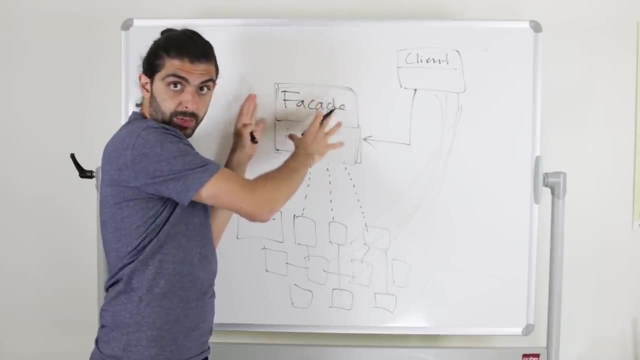 course make sense to interact with only one piece instead of interacting with all of these different pieces. That's really it. I mean, if you get that, you get façade pattern. So whenever you introduce a thing that you interact with instead of interacting with, 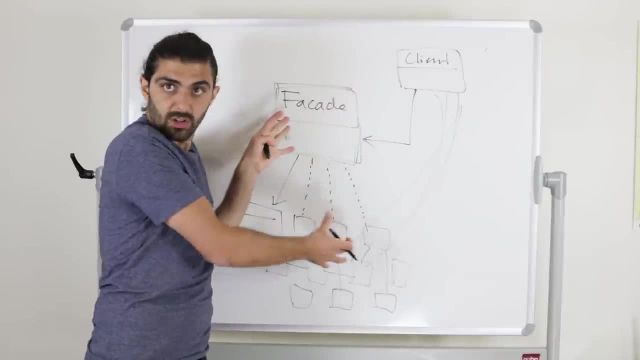 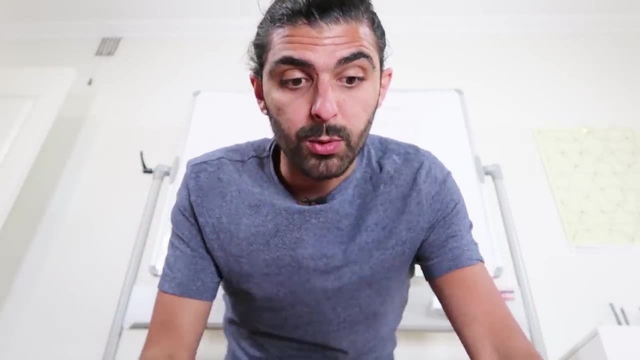 a bunch of different complex pieces. you've essentially used the façade pattern. That simple. Now, if you're not already familiar with this playlist or channel, what we're doing here is that we're walking through all of the patterns in this book: Head first design patterns, one by one, by one. 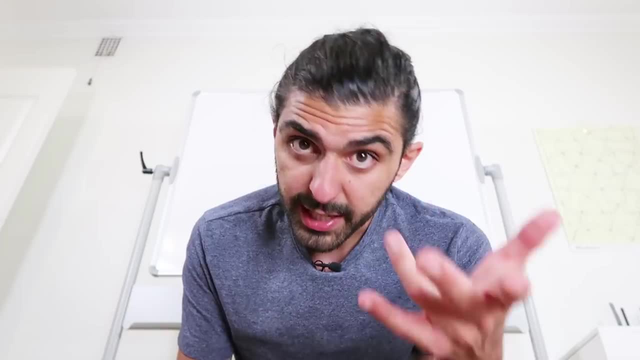 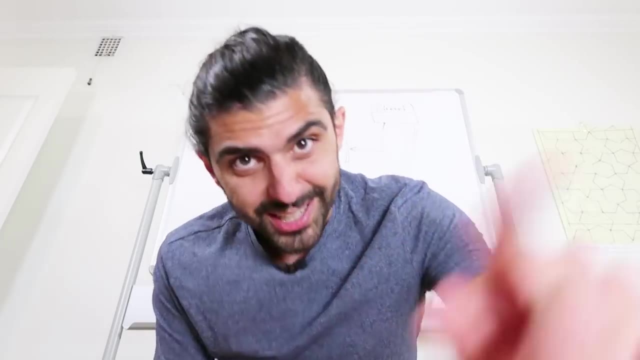 by one, And this is why we are now talking about façade pattern Again. next time we'll talk about proxy, and then we'll have a special video where we talk about the differences between façade, proxy, decorator and adapter, And then we're back to the regularly scheduled program where we go through the 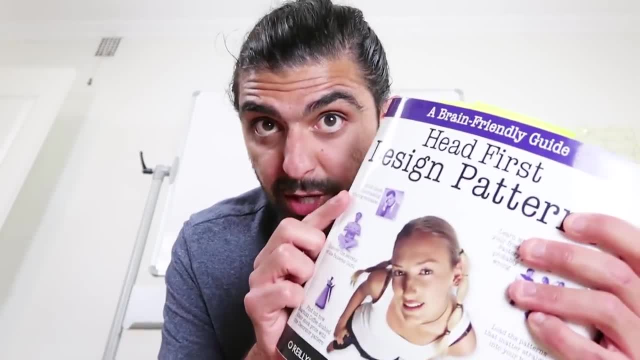 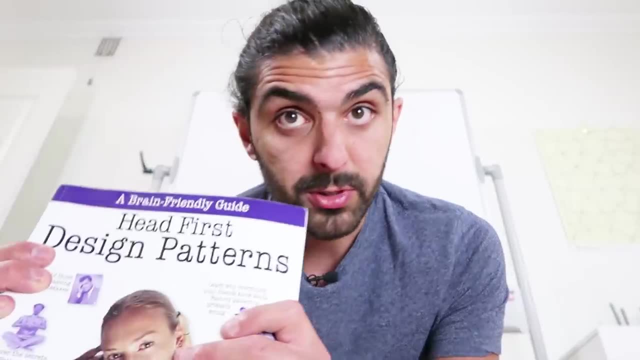 patterns of this book. Now, if you're new to design patterns, I would highly recommend that you get this book. Super pedagogical, It grows on me The more I interact with this book. I actually think it's kind of fundamental. I can really see why this has become sort of a course literature. 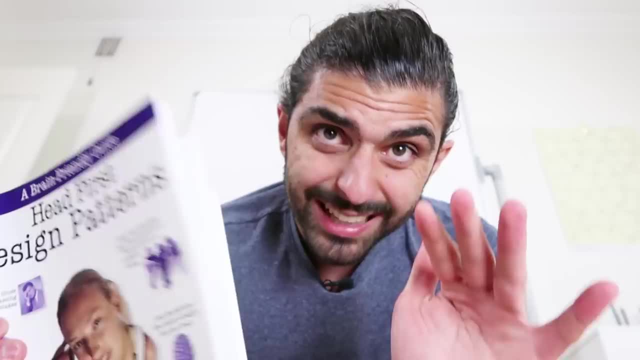 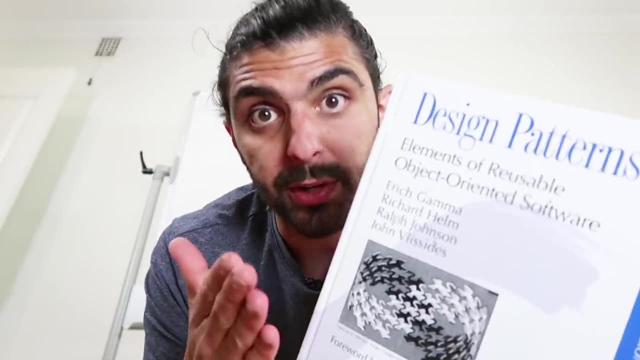 in a lot of courses Makes sense. Links are in the description. If you're not new to design patterns, I would rather say get this book instead. Design Patterns: Elements of Reusable Object-Oriented Software by Gang of Four. So this is like the classic de facto design patterns book. So put this: 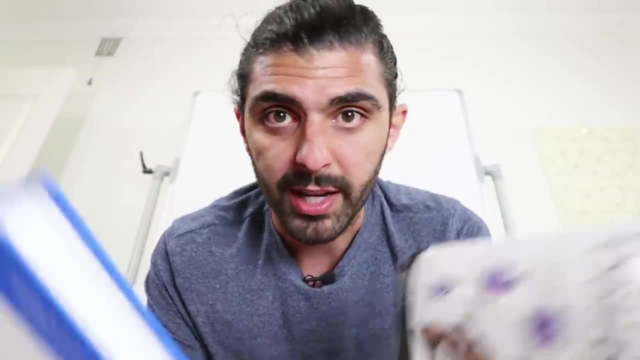 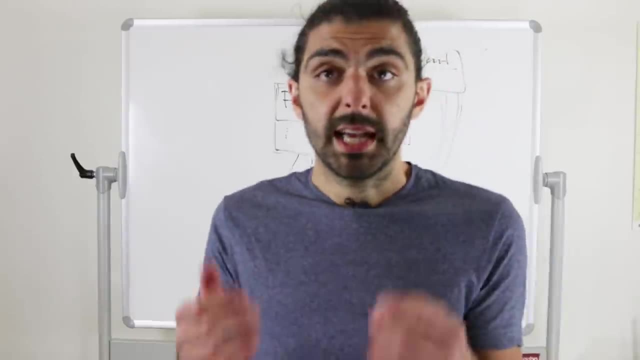 thing on your shelf and keep it as a reference. If you're new to design patterns, I would highly recommend it as a reference for the future. If you're like me, why decide? Get both? They're really good books. You'll learn from both of them. Links are in the description, Moving on, And actually we're kind. 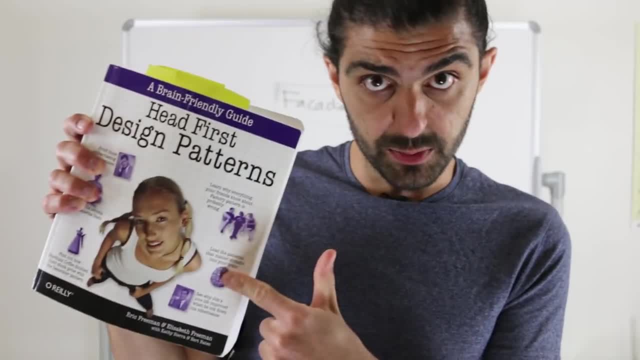 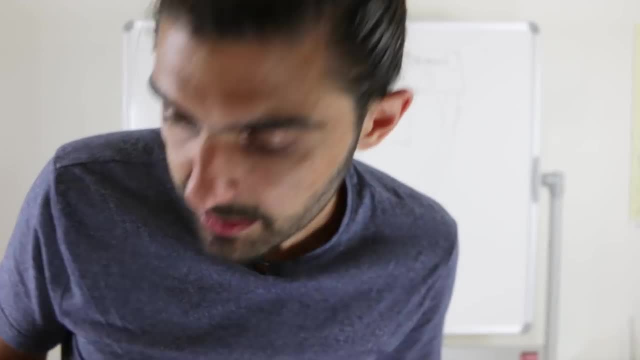 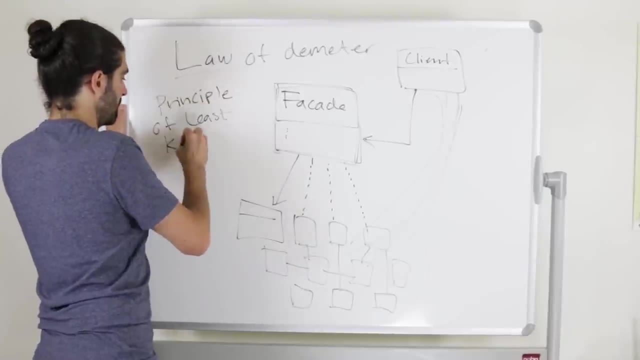 of done here. I just want to mention one thing before we move on. This headfirst book starts a discussion about the law of the meter, Law of the meter Zip, And apparently- I didn't know- it's also known as the principle of least knowledge. So the law of the meter. 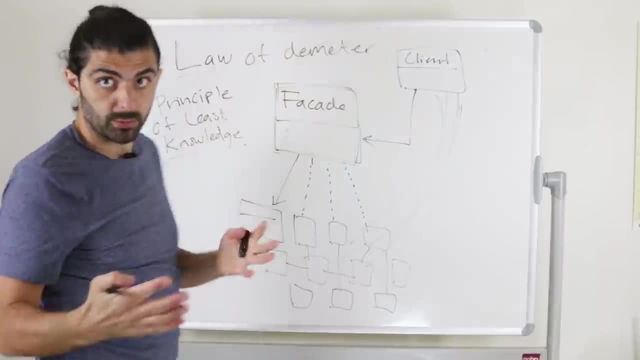 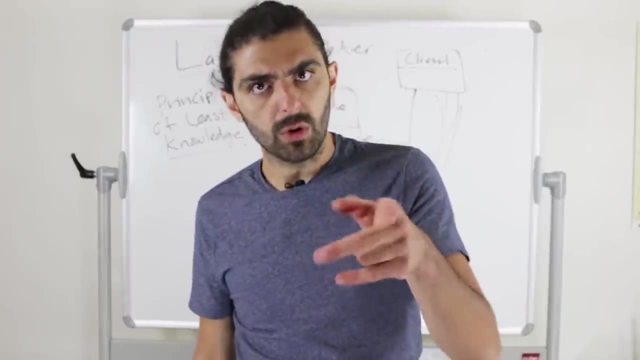 or the principle of least knowledge, In other words, the principle of knowing as little as possible. You can also think of it. I think it's often referred to as well as talk only to your immediate friends. Like objects should only talk to their immediate friends and not the friends of 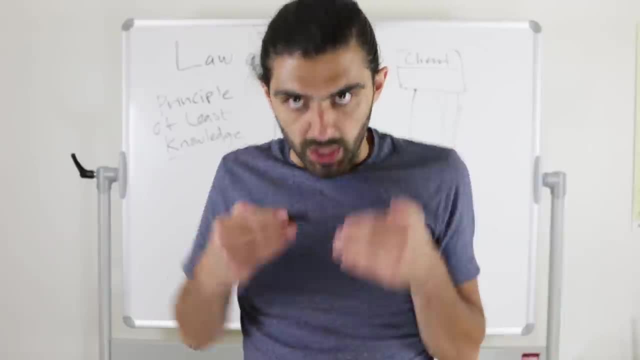 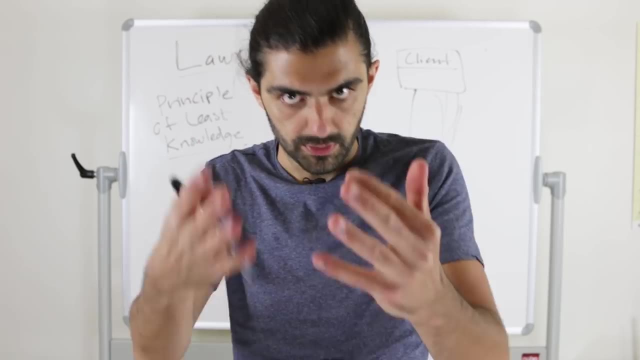 their friends Because of coupling. If you couple to only your friends, that's less bad than if you couple to your friends and the friends of your friends. Think about it: Coupling is bad because when we want to change things, it's very difficult to do so. So if you want to change things, it's. 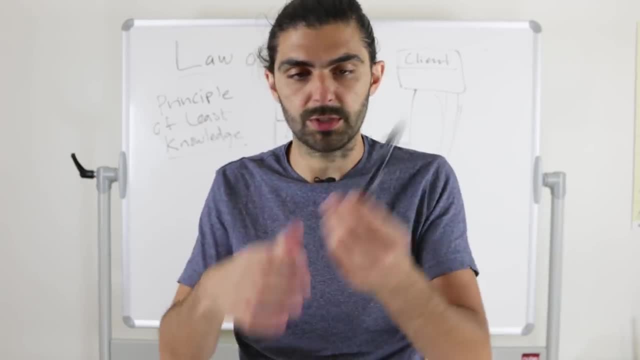 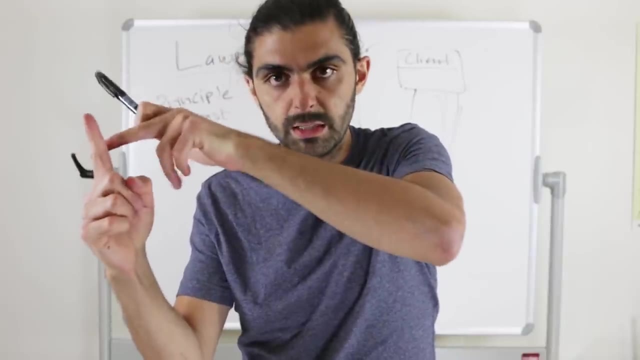 very difficult to change because things are coupled. In other words, if I have this thing and I have this thing and this thing couples to this thing and I want to change this thing over here, then the first thing might have to change as well, because this second thing has changed. 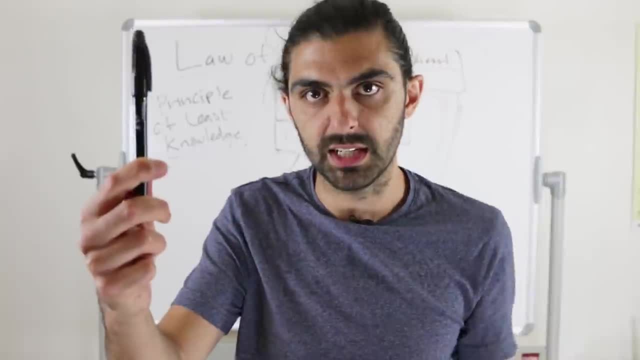 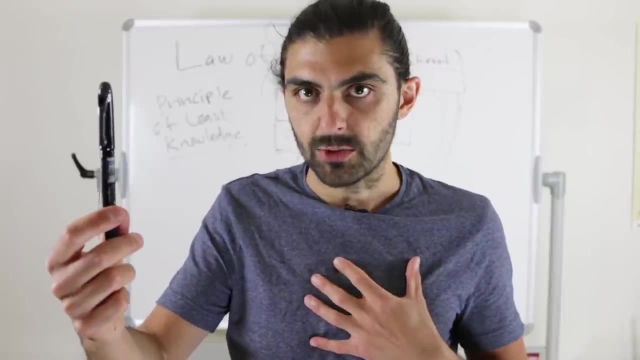 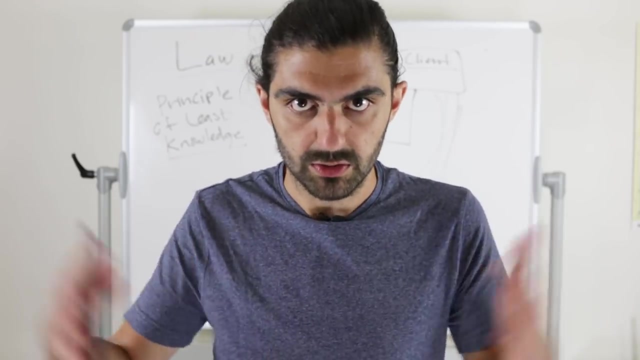 In other words, when the class representing me couples to this class representing the pen. if the pen suddenly changes in some way, the behavior of the pen changes, then I might have to change, because that change is not compatible with the way I was expecting the pen to work. And it's back to that old statement, like the sort of the golden grail. 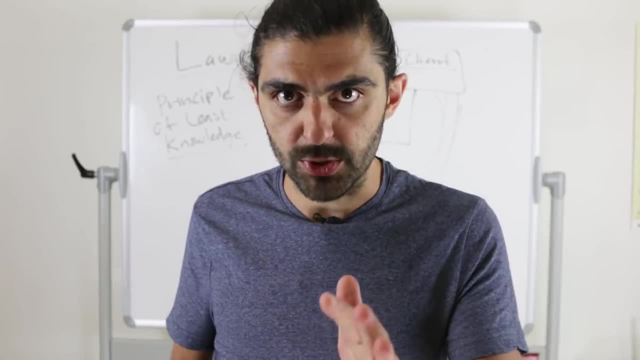 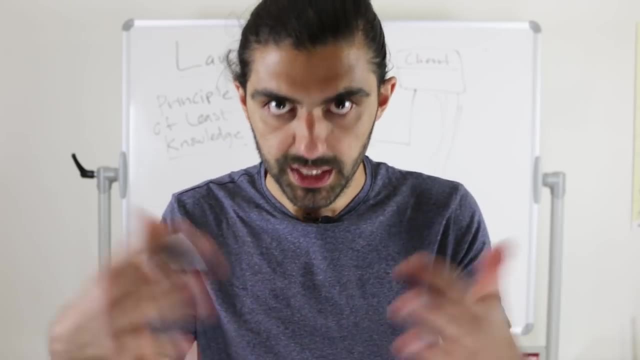 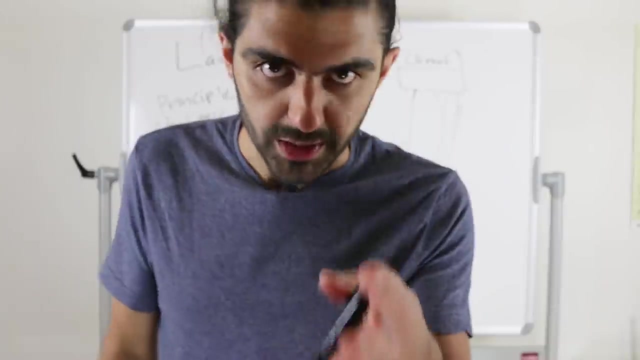 is low coupling and high cohesion, But that's a discussion for some other time. So, because of coupling, law of the meter or the principle of least knowledge or talk only to your immediate friends, those are rules that are introduced as an attempt to make us reduce coupling. But what? 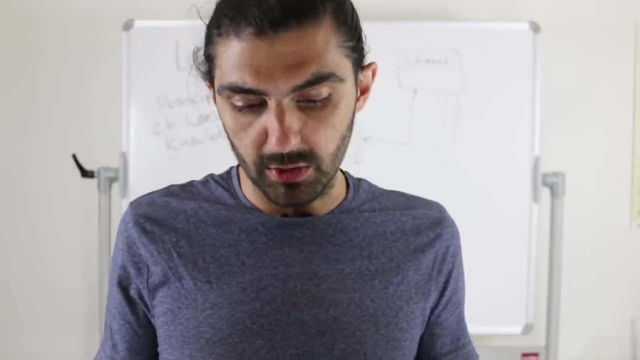 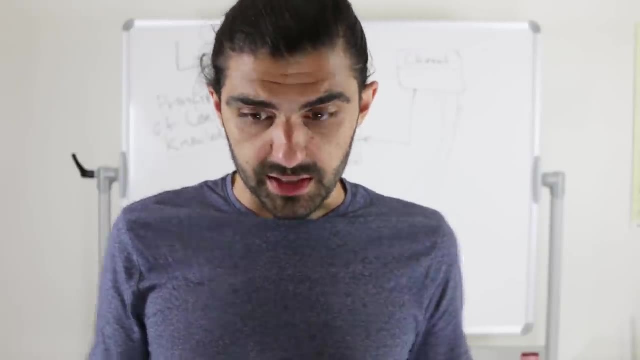 do they actually say So? in this book there's this list of which methods are allowed to be invoked when you are in a relationship with your partner and which methods are allowed to be involved when you are trying to follow the law of the meter. Actually, this is quite interesting. 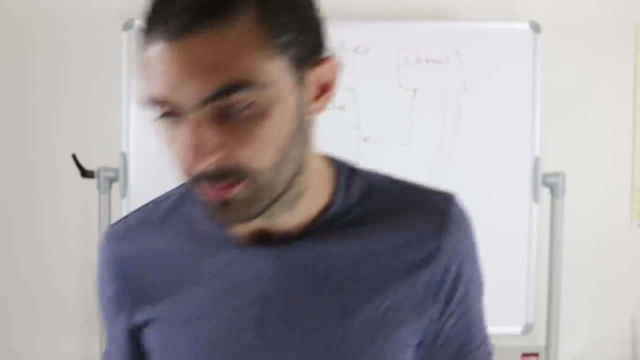 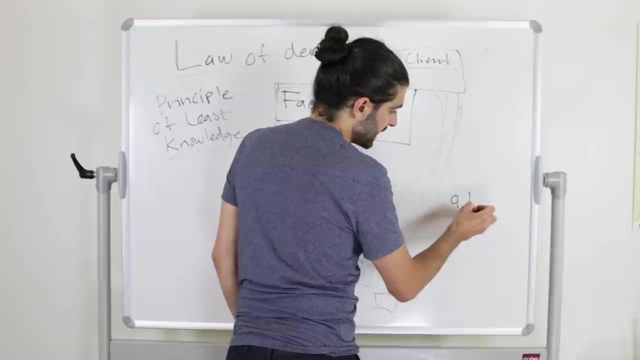 because I had learned it in a much more sloppy way. Let me just give you the sloppy way first. So the sloppy way is this: that you're only allowed to say a dot B and you, but you're not allowed to say a dot B, dot C. So you're allowed to say a dot B, but you're not allowed to say a dot B, dot C. 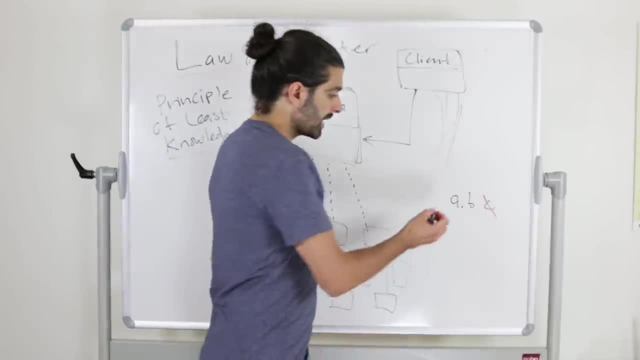 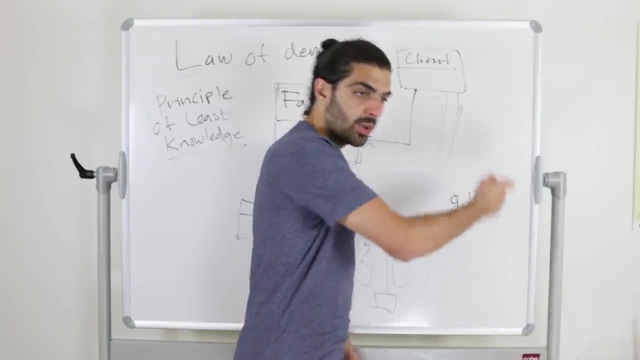 And that's sort of the naive explanation, which means that you're allowed to talk to yourself, you're allowed to talk to things that you know, but you're not allowed to talk to things that things that you know know. You're allowed to talk to yourself. you're allowed to talk to friends. 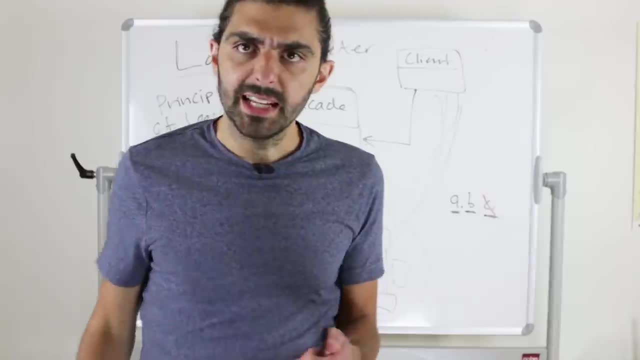 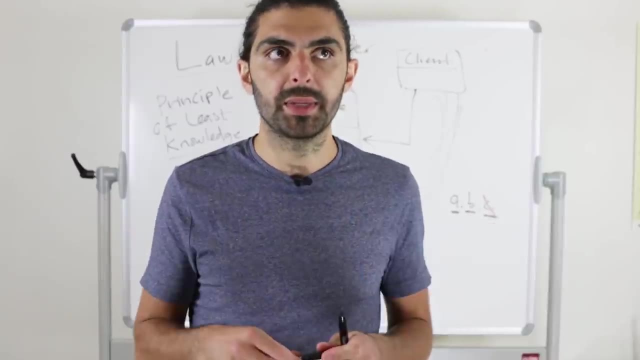 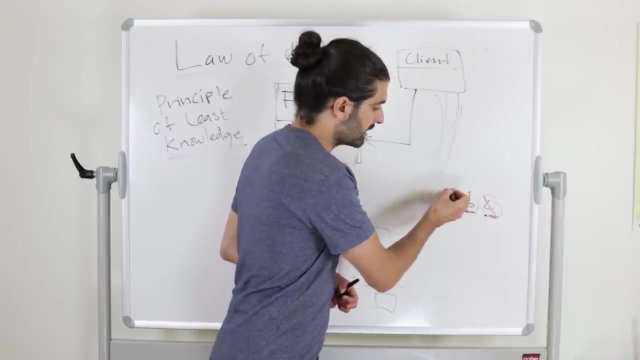 but you're not allowed to talk to friends of friends, And I think this is summed up quite well in the statement that following this kind of logic leads to interfaces that are wider, because if B is supposed to act on the on behalf of C to A, that means that 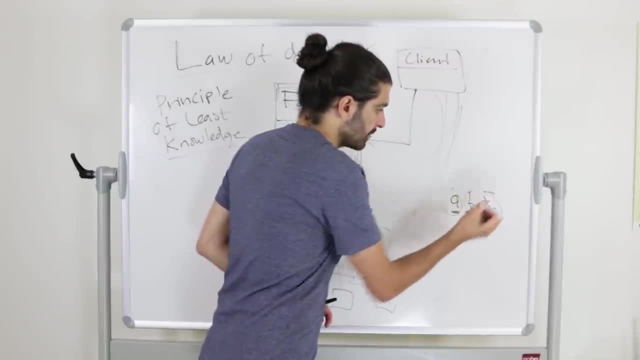 B needs to kind of implement the interface of C if A wants something from C and B has C. So it's like instead of A calling B and getting back a C and then calling something on C, it's like A calls B, who calls C and then gives something back to A, which might mean that B now 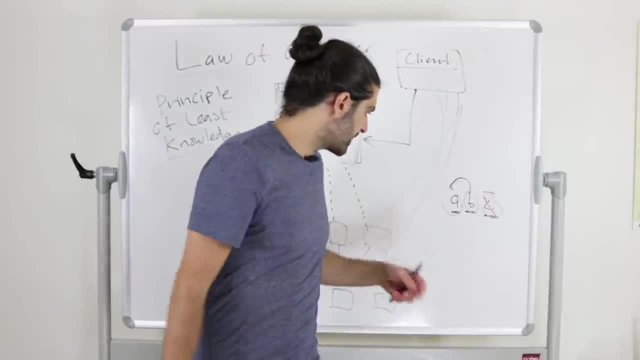 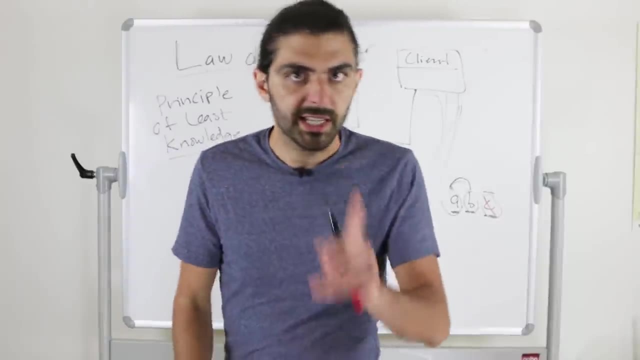 has to broaden its interface. But I guess the point is that if that happens, that means that B has too much responsibility or something along these lines. But I really don't want to dig in here. I just want to point out that there is some controversy here And, if you're interested, please 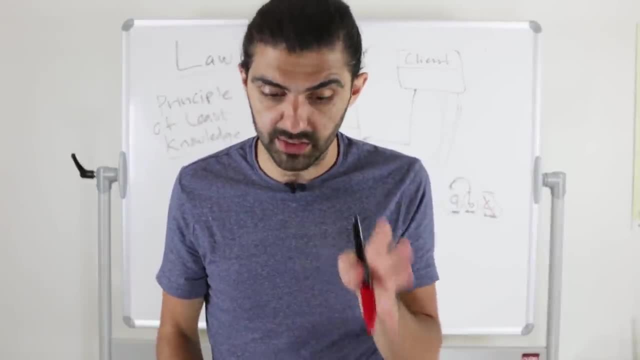 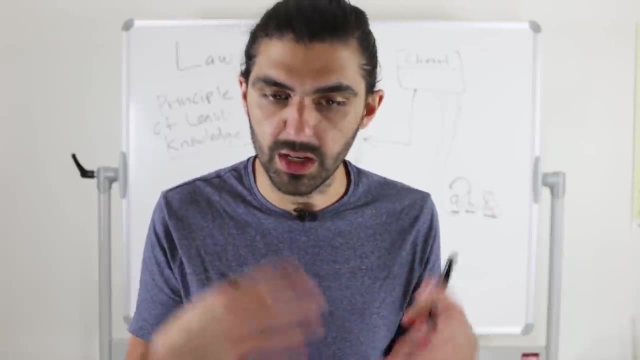 let me know in the comments and we'll definitely dig down here, because I think there's probably a super interesting discussion here. I mean, it seems that this has more to do with types rather than the number of calls or something along these lines. So you already know that I recommend you to. 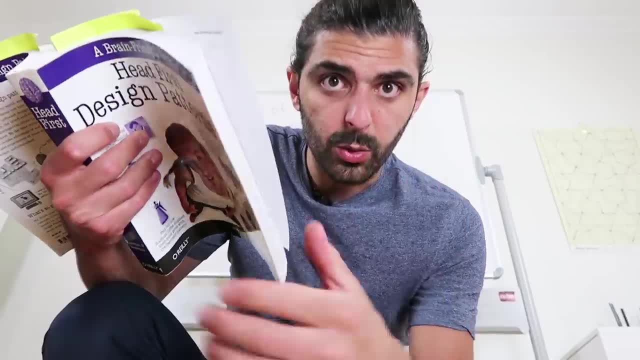 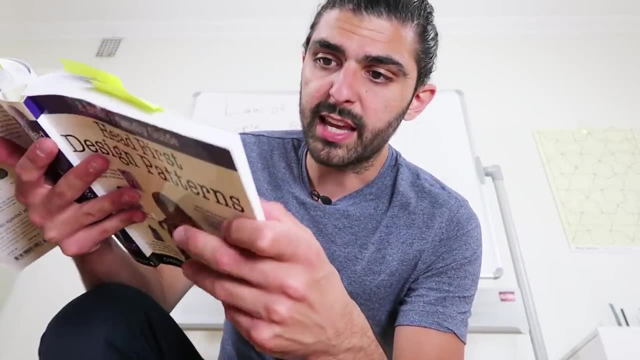 get this book if you want to know more about design patterns. But if you're interested in the law of the meter discussion, I actually think it's a good idea to get this book as well. So when I said ABC, what they say is that they have this definition. They say that if you are in a 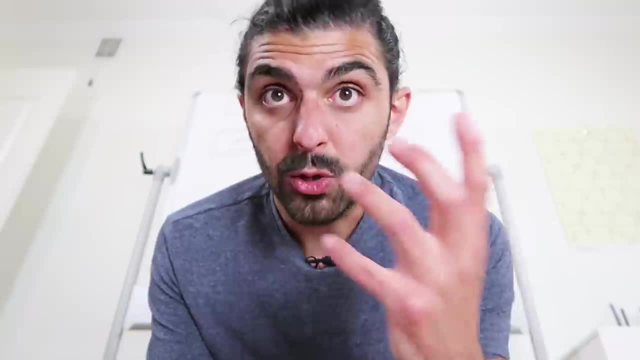 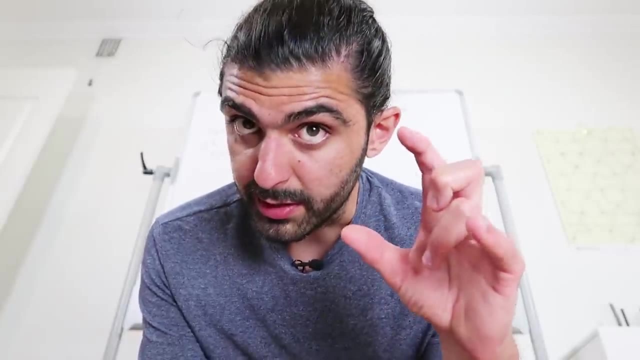 particular method in a particular method. if you are in a particular method, in a particular method in a particular object, you're only allowed to invoke some particular methods. It depends on where these methods reside. Imagine that you're in a method in some particular object. You're only. 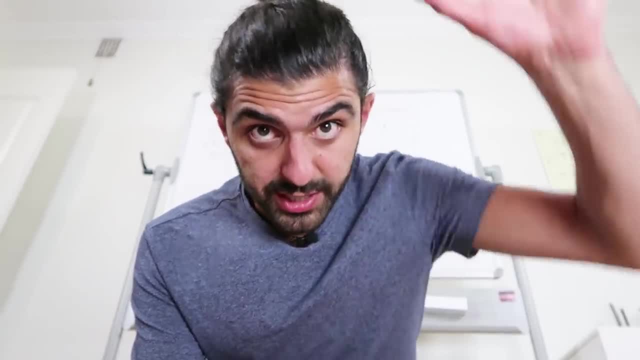 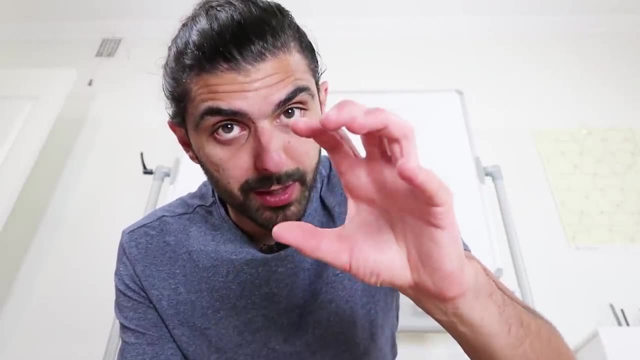 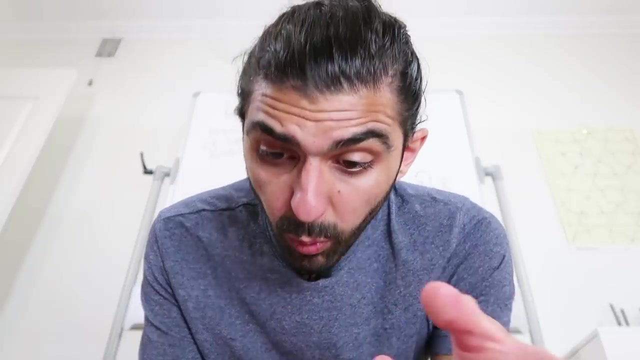 allowed to invoke methods on the object that you're in or objects that have been passed to you as a parameter. So you're in a method, you've been passed some particular parameter and you're allowed to invoke methods on that parameter. Or third point, 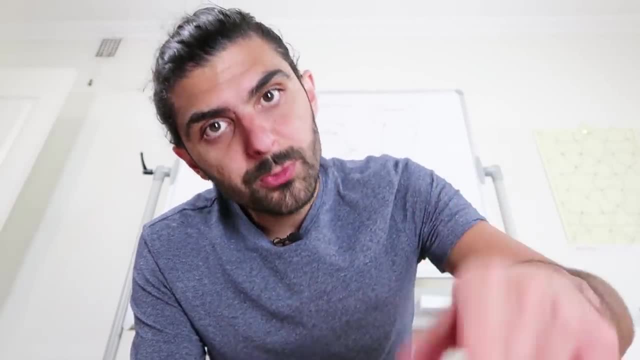 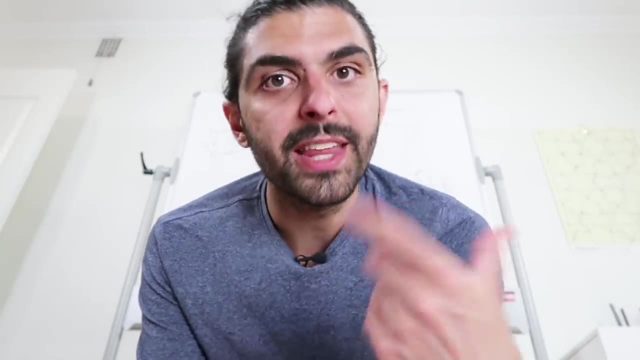 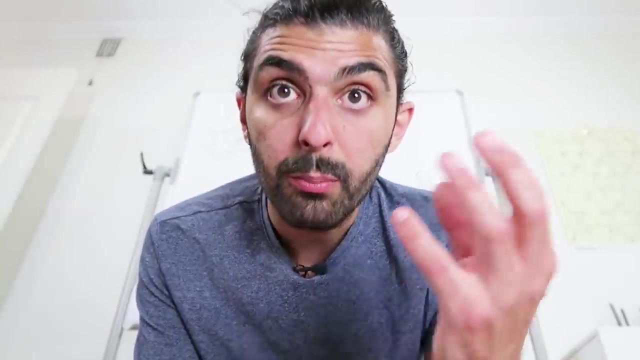 you're allowed to invoke methods on objects that you've created yourself. So if you're in this method and you've created an object, then you're allowed to invoke methods on that object that you created. And fourthly and finally, you're allowed to invoke methods on a component of this object. 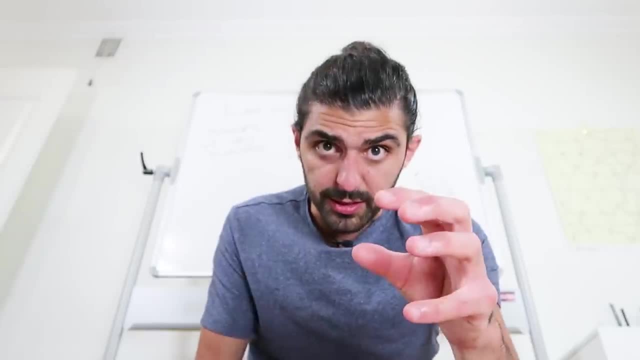 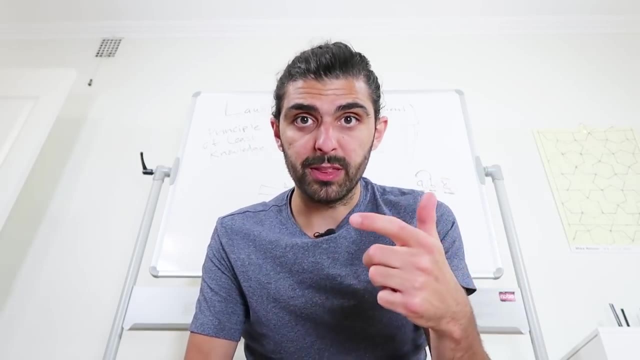 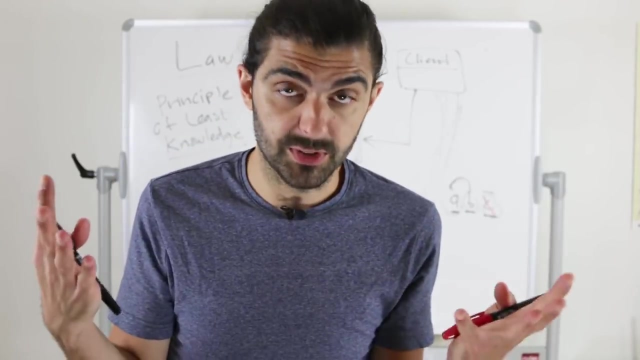 which means, for example, an instance variable. So if you're in a method and that method's in a class and that class has been instantiated and then you have an instance variable, you're allowed to invoke methods on that variable. And I don't think I've covered these more than 10 times. 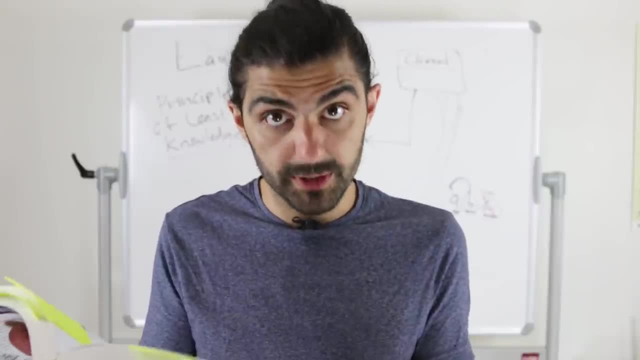 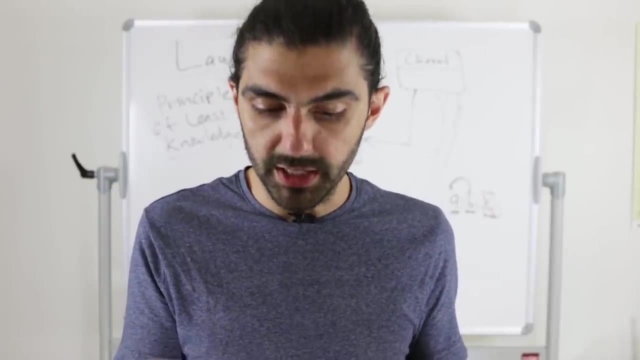 But let's leave that aside. Regarding the facade pattern, I think we've nailed the facade pattern. The only thing missing, which I forgot before, is actually the definition, So the definition of facade pattern. from headfirst design patterns, The facade pattern provides a 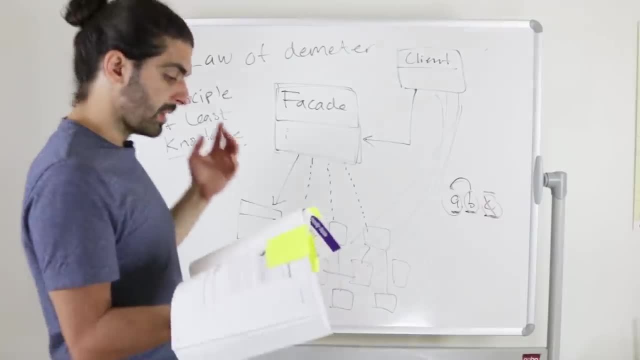 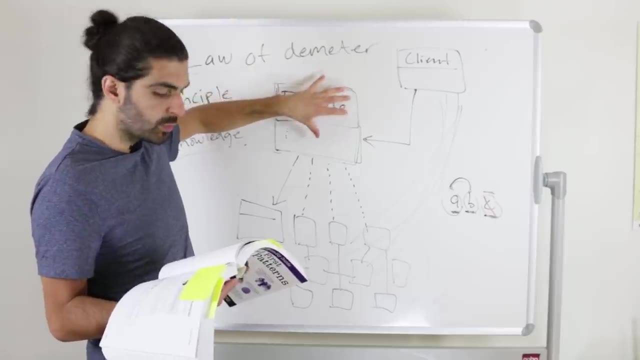 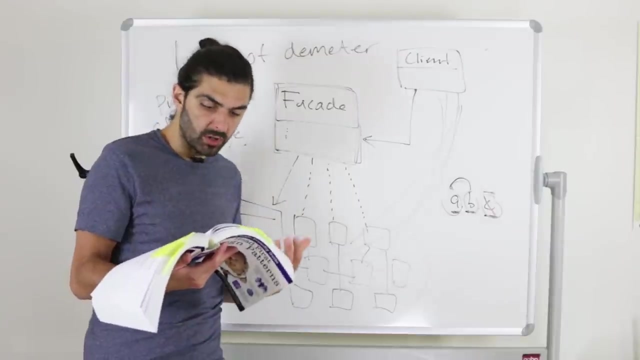 unified interface to a set of interfaces in a subsystem provides a unified interface- that's the facade which is used by a client- a unified interface to a set of interfaces. this set in a subsystem Facade. then it's like an explanation Facade. 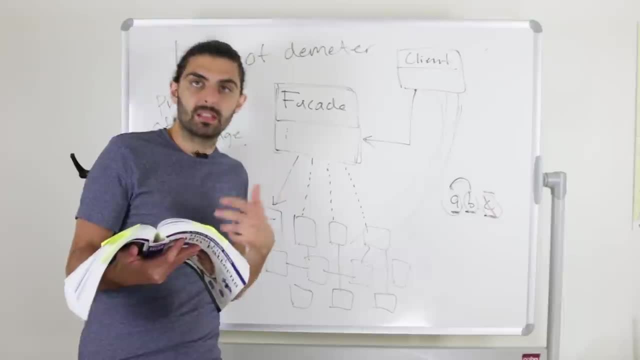 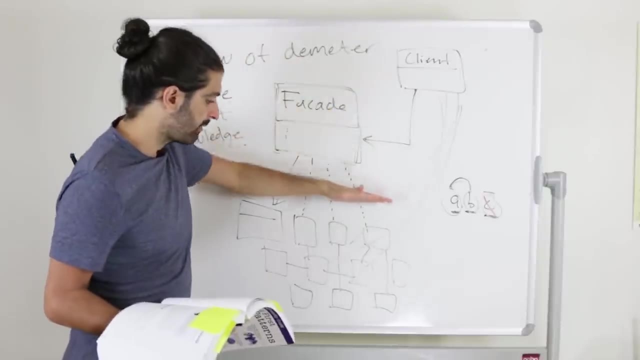 defines a higher level interface that makes the subsystem easier to use. So it's not like it's adding additional functionality, It's just on a higher level. It's like we have all this complex stuff here and instead of interacting with that complex stuff, we have this higher level facade. 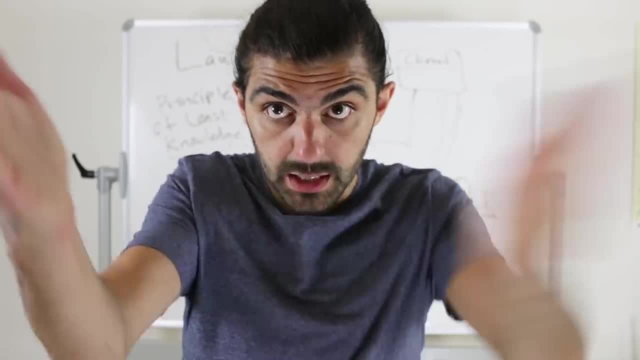 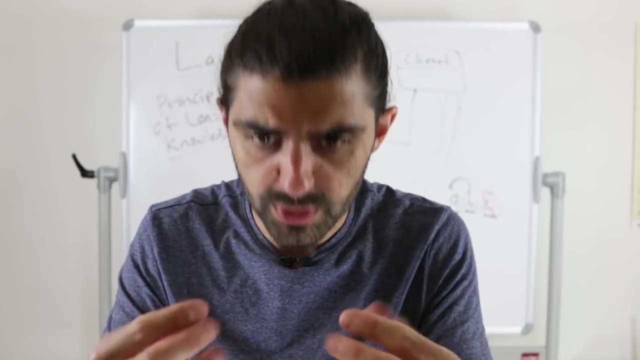 that we can interact with instead, And that's it. Beyond that, links to both these books are now in the description. You now know the facade pattern. If you don't, or if you found this confusing, or if you have anything you want to add or some examples or anything that you want to talk about,